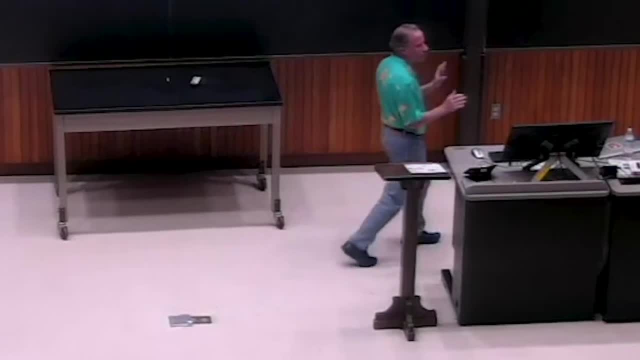 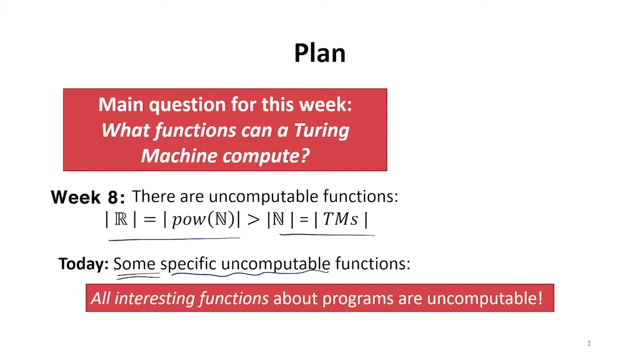 a bunch of different kinds of numbers and shows that those are computable, to give you a sense of- yeah, it seems like we can actually do what we want with this kind of model. Today we're going to get to see some specific examples of functions that are not computable. 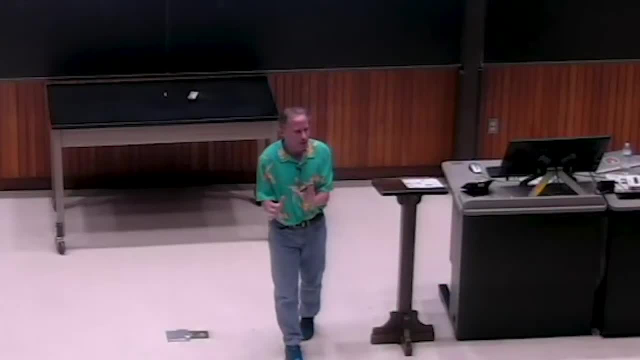 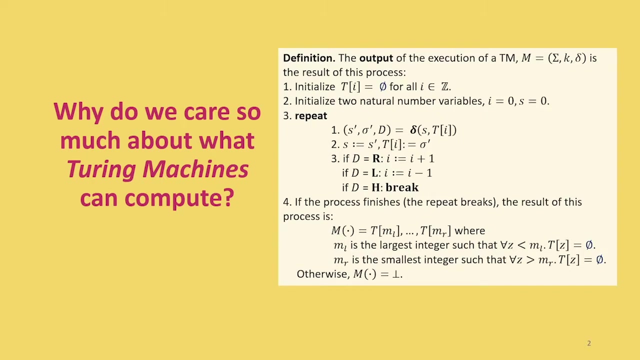 And we'll actually not just see some. We'll get to a very strong result. that is basically every interesting function that we might want to know about. a program is uncomputable. Why do we care so much about what Turing machines can compute before we actually get to what? 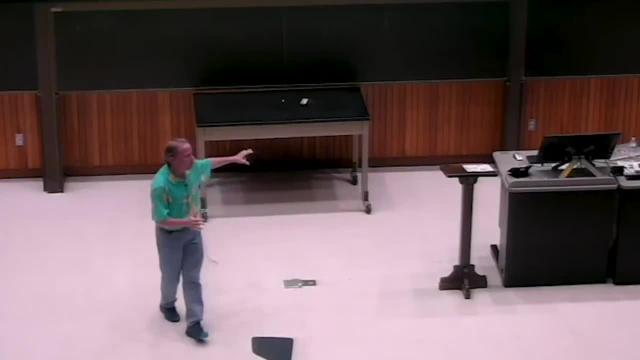 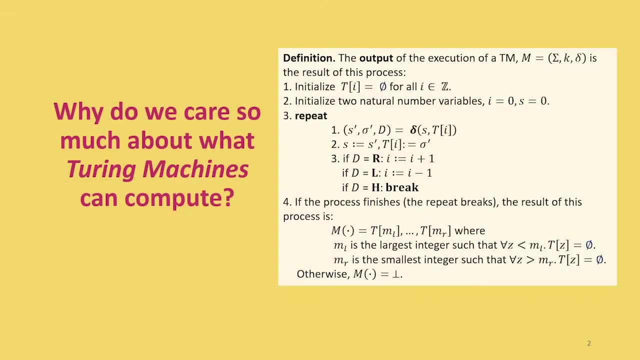 they can't compute. We define this very specific model and we're asking and answering these questions about a specific model. And not only that: the actual model that we talk about keeps changing because the book is getting updated. The real question is: what's so special about Turing machines? 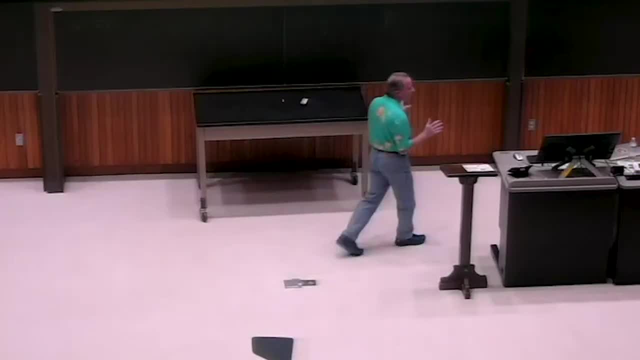 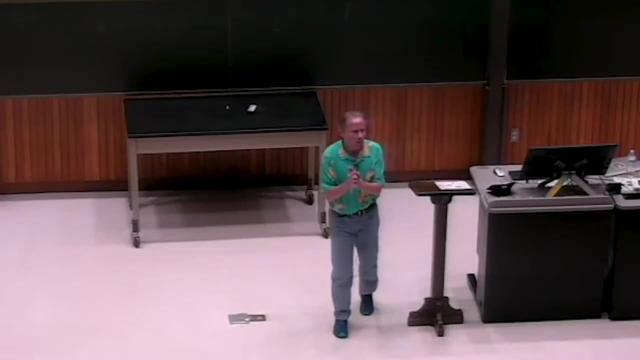 We could think of lots of different models, And what's special about Turing machines is that our reason for thinking about these models is that they're actually all the same. All models that have any semblance of what we might think of as a computer seem to be. 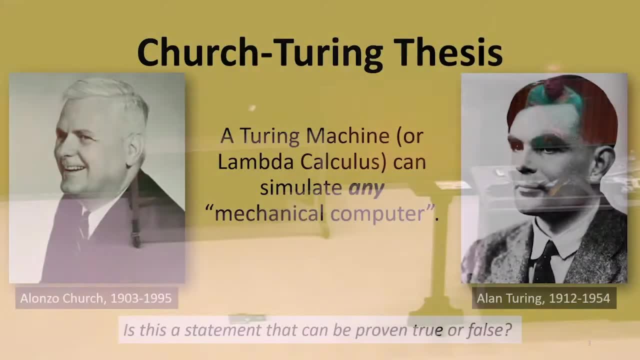 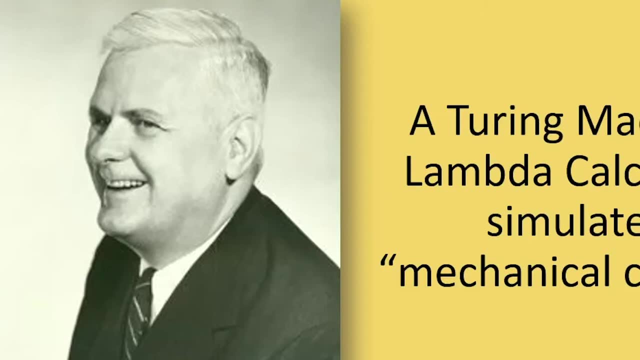 equivalent to Turing machines. So this is actually what's called the Church-Turing thesis. It's a name for Alonzo Church, who we haven't talked about much yet, But around the same time Turing was coming up with Turing machines, Alonzo Church came. 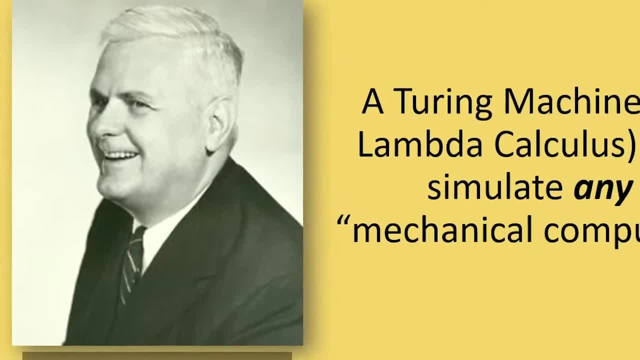 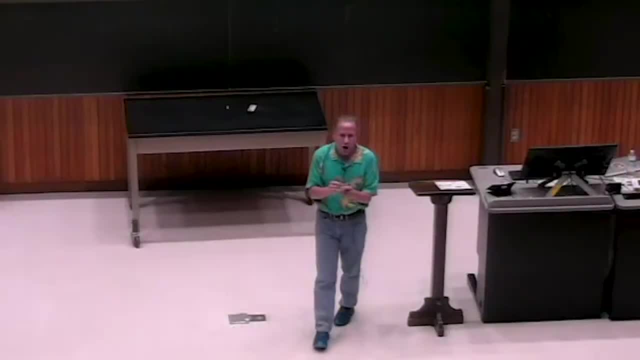 up with lambda calculus, which you've used, at least in Python. the lambda expression comes from that And he answered the same question Turing was trying to answer with his Turing machine model about this question about things that are decidable. that came from Hilbert's problems. 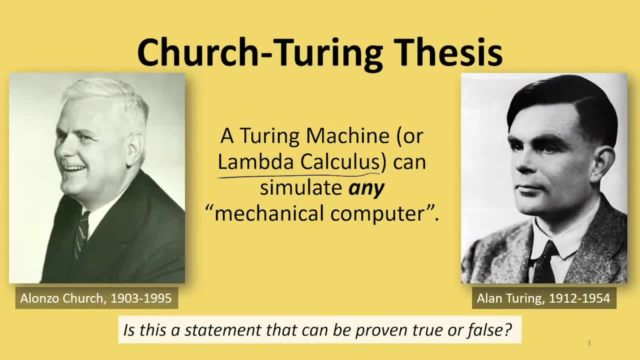 And he solved that by inventing lambda calculus and showing that that seems to be a model of computing that's useful and there are things that it can't do. And Turing established this Turing machine model that we've been talking about And it turns out those are equivalent and what either one of those models can do is 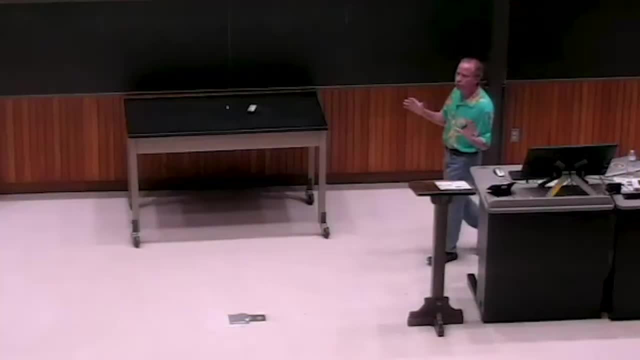 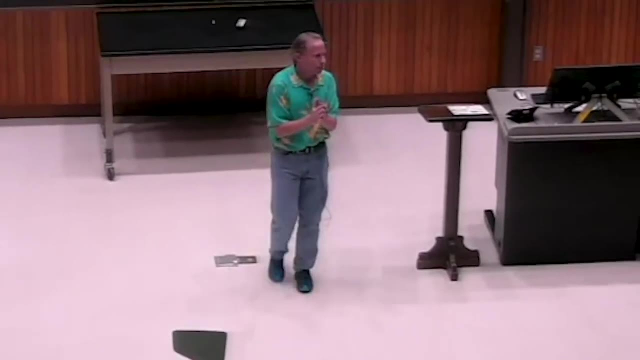 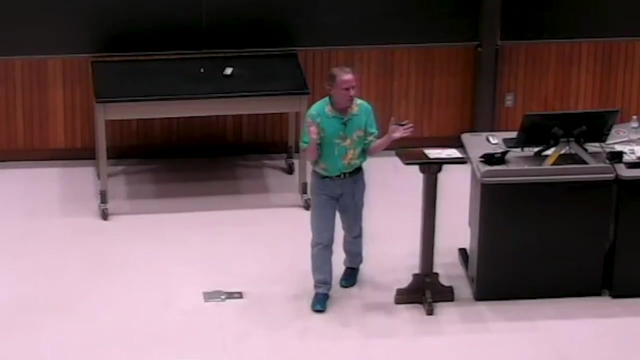 simulate any mechanical computer. And that's basically the Church-Turing thesis, to say that this model of computation is powerful enough to simulate all other models of computation. So this is called a thesis, It's not called a theorem. So if it was a theorem that would mean we should have a proof. 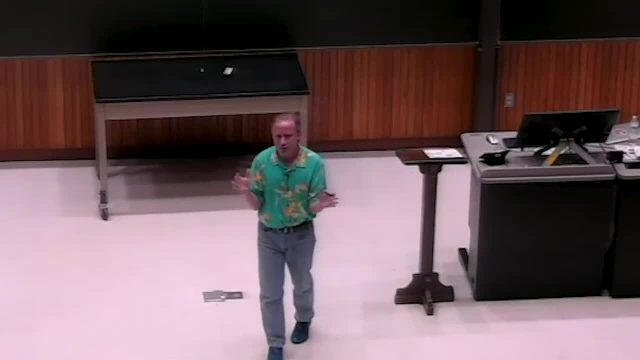 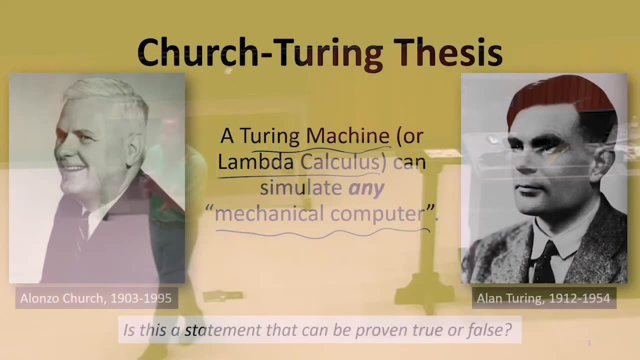 If it was a conjecture, it means, well, it's something, a proposition someone has stated but we haven't been able to prove yet. But this is called a thesis. So why is this a thesis and not a theorem? Is this something we should be able to prove? 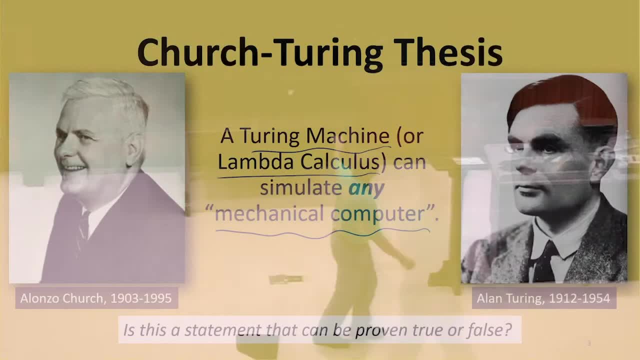 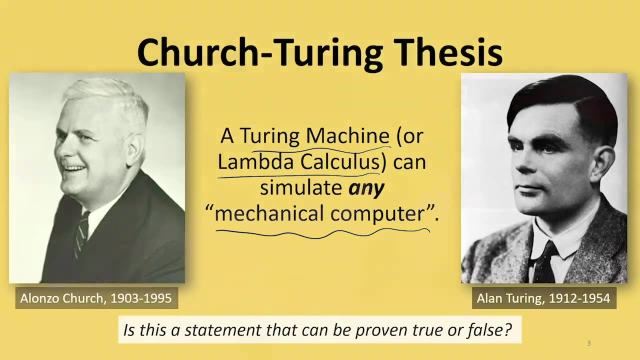 Should we be able to prove if we tried hard enough. This is really a claim about something that we haven't defined. So for any defined computer, well then we should be able to have a concrete proof that says whether or not this is as powerful as a Turing machine, or more powerful, or something. 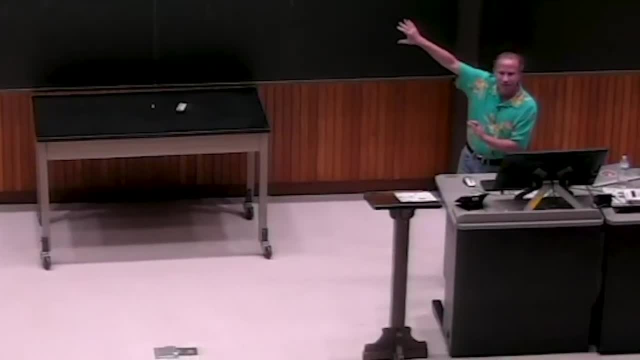 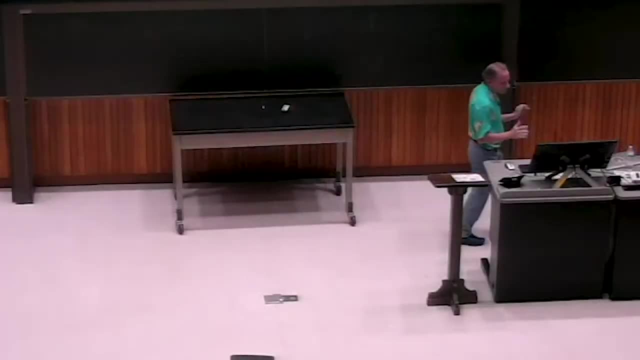 else. For any concrete model of the computer that we define, well, then we should be able to have a proof that says whether it's equivalent or not. You'll do lots of problems like that, But this is stronger than that. This isn't saying for some specific model. 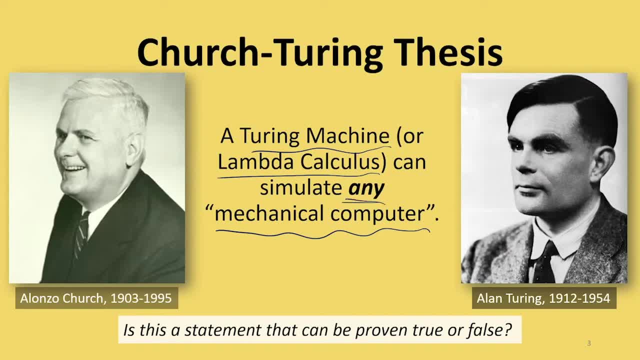 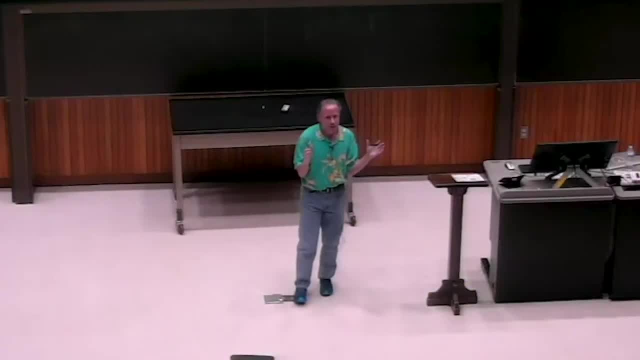 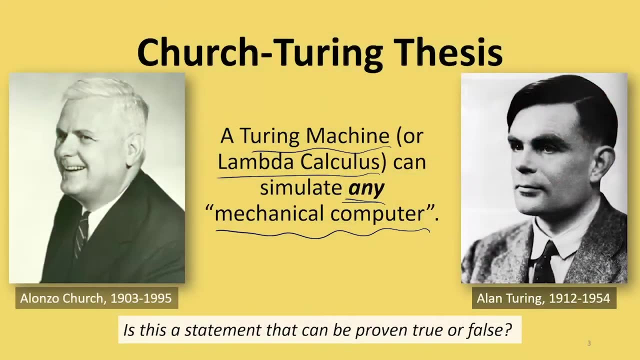 This is for any model in this large, vaguely defined class that we can't even define, but something that corresponds to our notion of what we think a mechanical computer is. So that is not a defined mathematical object that we can prove things about. It's something much more intuitive than that. 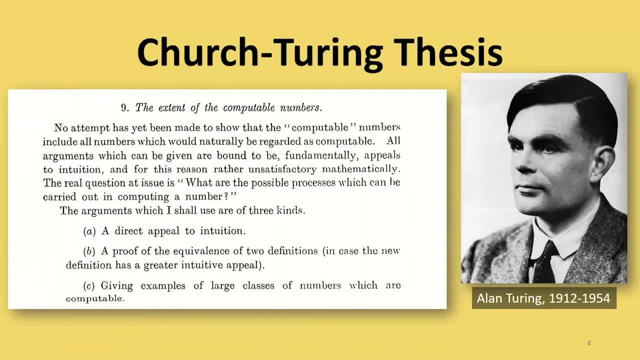 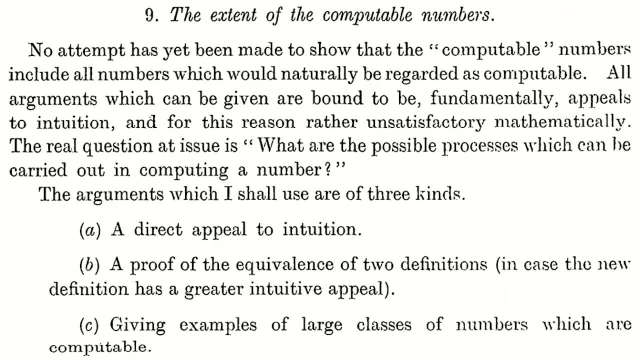 If you read Turing's paper, which you're not really assigned to read, but I hope all of you will read at some point, maybe not this week. he makes this argument And it's pretty nice the way he makes it. So there's computable numbers. 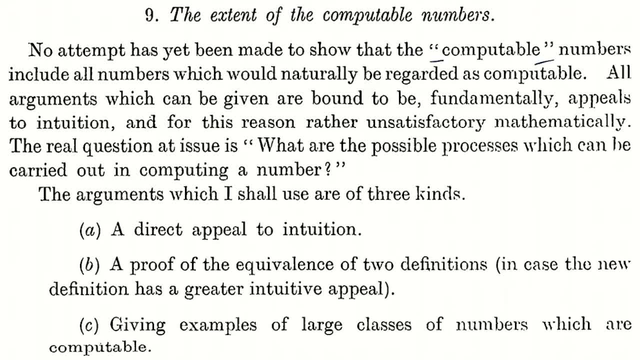 Which is this notion? the question of what numbers can be computed by finite mechanisms. well, that wasn't stated as what can a Turing machine or what can some specific formal model of computing do? It was stated as things that can be computed by finite means. 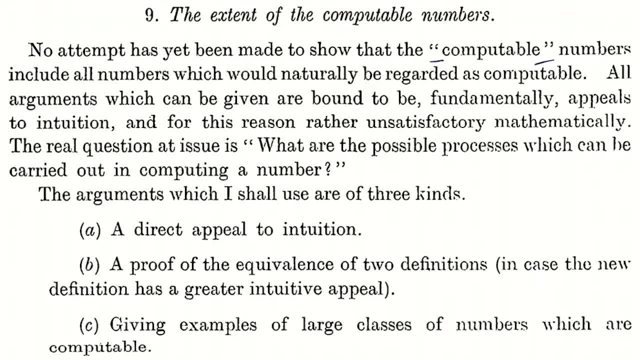 That isn't defined what we can actually use to compute with. And so he makes this argument that, well, we're going to claim that the model actually covers everything that we could reasonably think of as being done by a computer, And he makes that three ways. 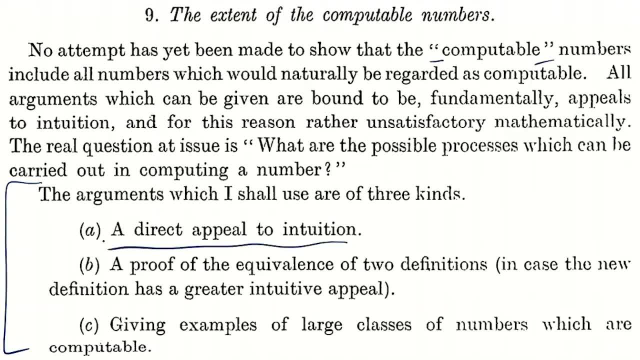 So he makes an appeal to intuition. Certainly that's not a mathematical proof. He says: for some specific definitions we can prove their equivalent. But that doesn't cover the whole thesis. That just says these specific things that seem like they're really different, and certainly. 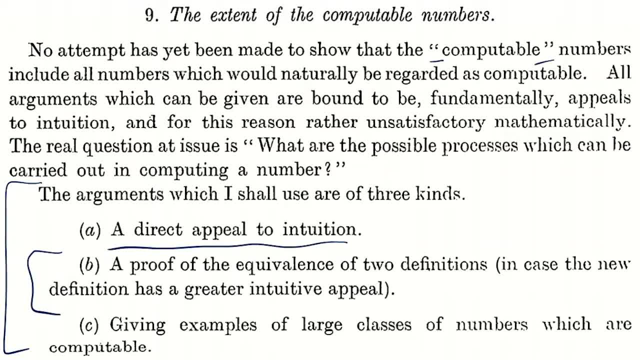 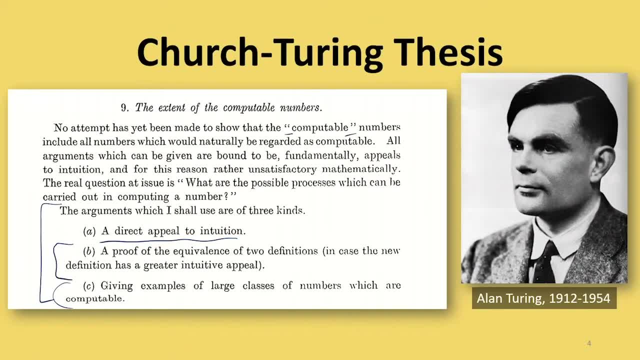 lambda calculus and Turing machines seem really different. we can show their equivalent. The third thing is: well, we can look at lots of functions that we think we should be able to do and show that our model can do them. Or, in this case, look at the model. 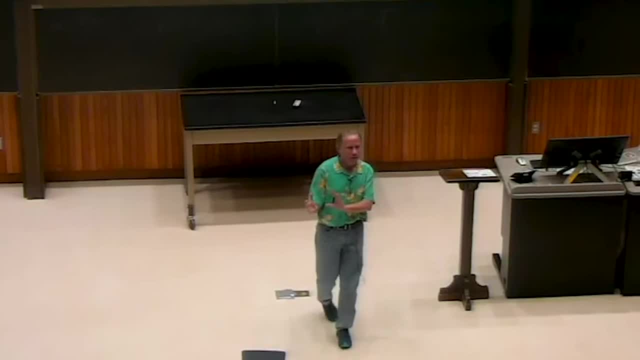 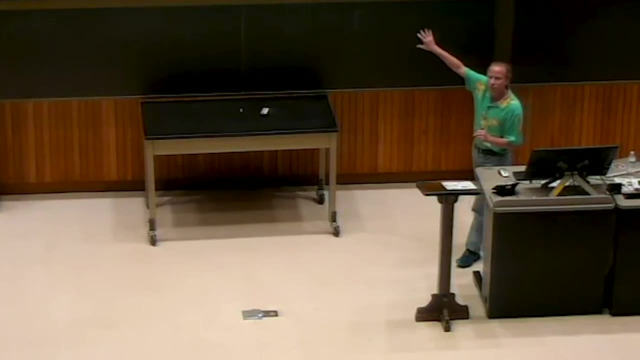 We can look at lots of numbers that we think we should be able to compute and show that we can do them. All of those are things that are meant to build confidence in this intuitive, fuzzy argument that everything that we can imagine as a mechanical computer can be simulated. 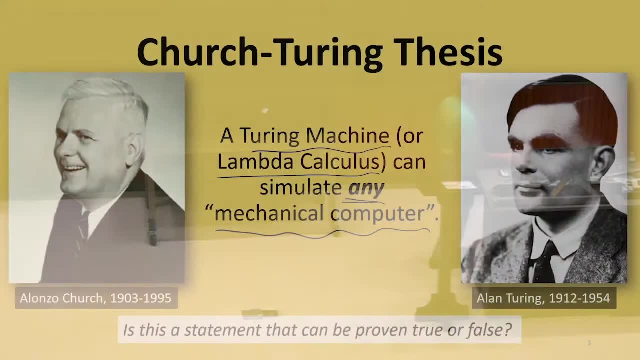 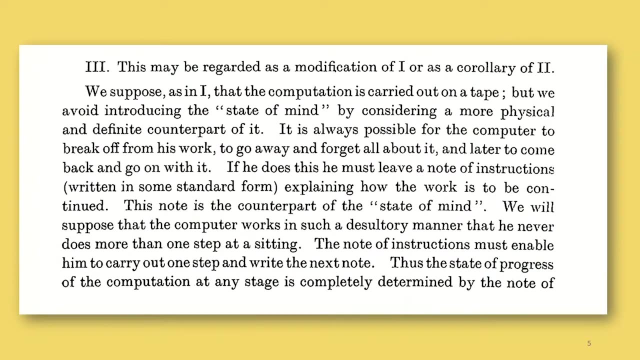 this way or is equivalent in power to this, But it's not something we can ever prove Part of. this intuitive argument is also connected to the simulation argument for specific things. So one of the things he argues which I think is pretty neat is- and we talked about sort- 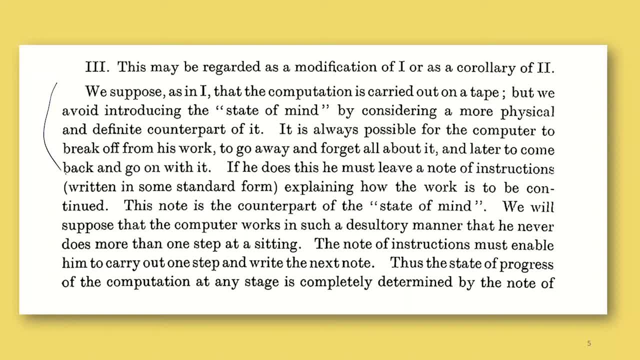 of why finite number of states. Well, maybe human computers can do more than that, Maybe they can keep track of something else, And he argues that well, any model that wouldn't account for. maybe the human computer can leave in the middle of a problem and go have dinner and come back, and they better be able to. 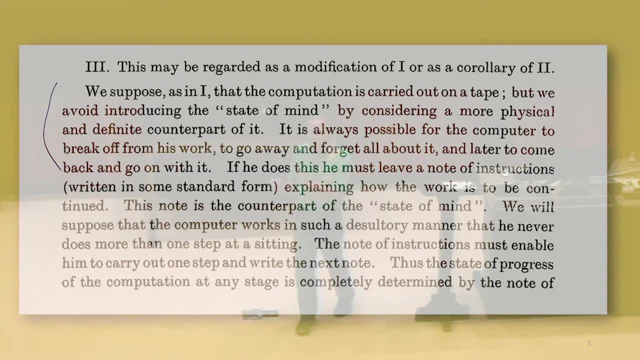 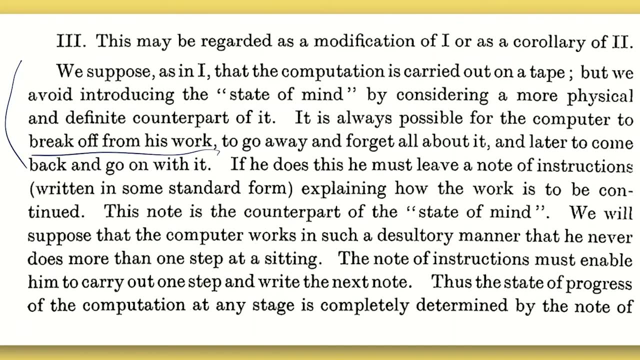 continue where they left off and not make a mistake or not lose track of the problem they were solving. Any model that can't account for going away and having a break doesn't seem right. If we account for the human, computer should be able to take a break. that means everything. 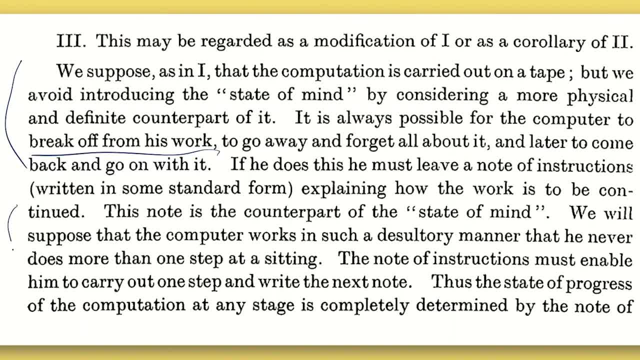 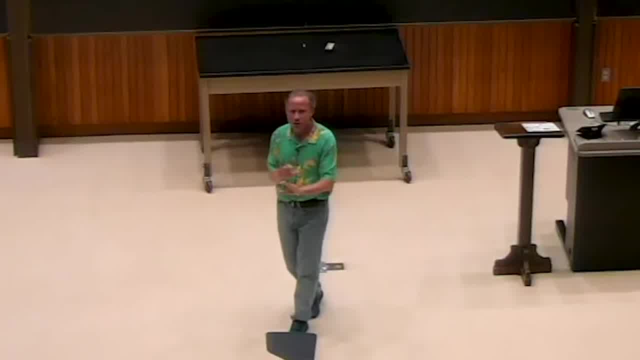 that they need to keep track of To be able to continue has to be something they can write down in a finite, simple way. That's a very intuitive argument. You could argue that well, the human computer shouldn't get to take a break, and there might. 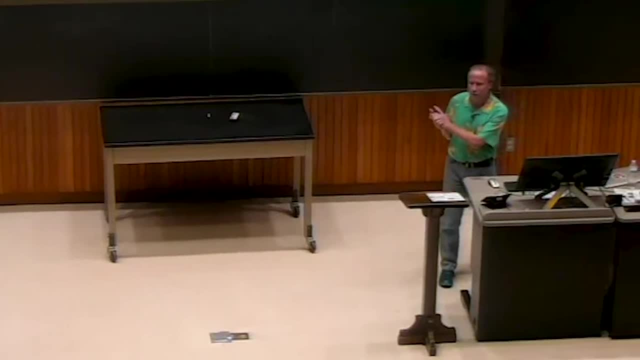 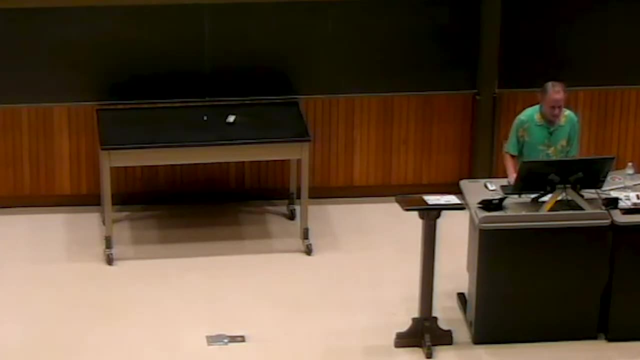 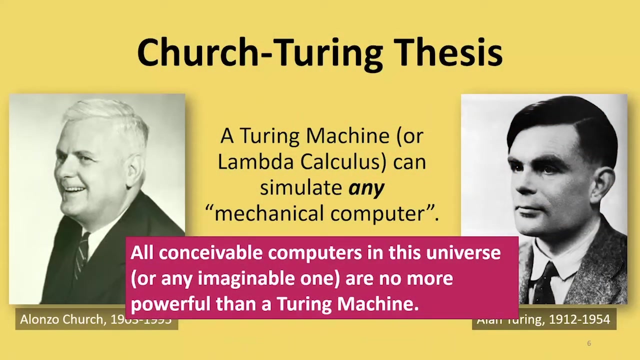 be something they can keep track of in their head that you couldn't keep track of with a finite state. But that's just an intuitive argument that the things that we can think of computers doing we can model this way. So what the result of this is informal notion of we can simulate any mechanical computer. 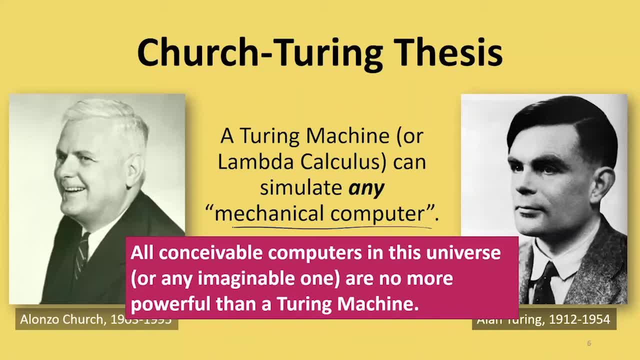 with a Turing machine. If we can simulate any other computer with this one, that means that this one is at least as powerful as anything it can simulate. So that is making this very strong claim which again is based on this informal notion. 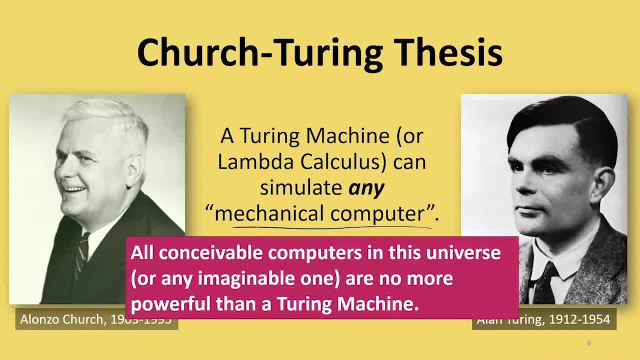 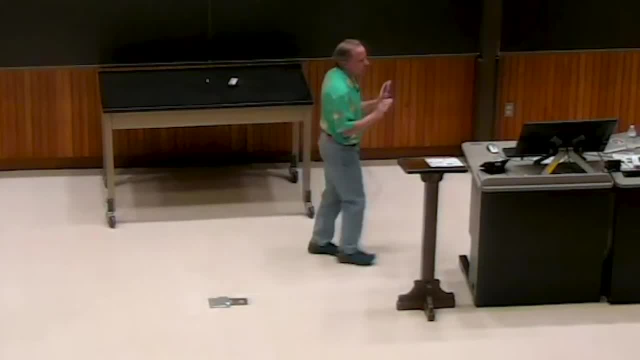 of what mechanical computers are that? all conceivable computers in the universe that we know, and probably any other universe we can imagine, are no more powerful than a Turing machine. So if we can find things that a Turing machine cannot compute, that's a really strong result.